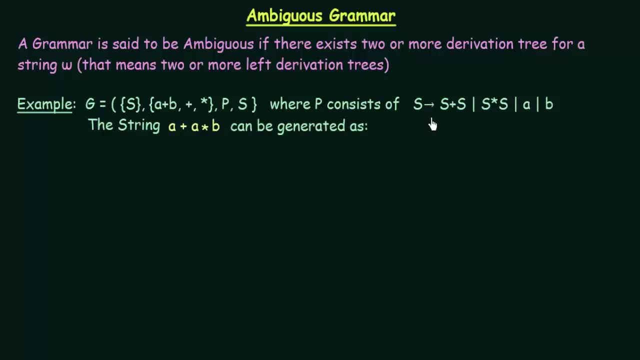 And the production rule is given like this: S gives S plus S and S can also give S into S, and it can also give A and it can also give B. Now we want to generate the string A plus A into B. This is the string we want to generate and let's see in how many ways we can generate this string. 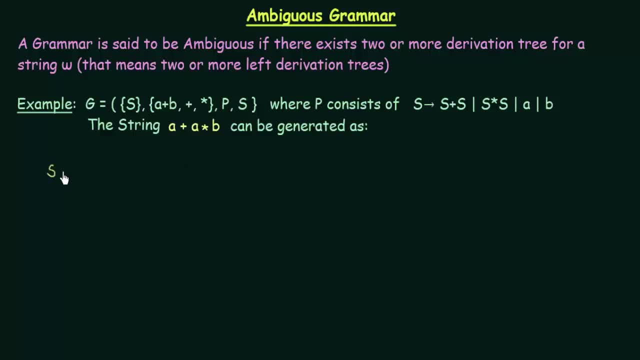 Okay. so let us start with the start symbol, which is S, and I will say that S gives S plus S. I will start from this production: S gives S plus S, S plus S. Okay, now I need to get A plus A into B. 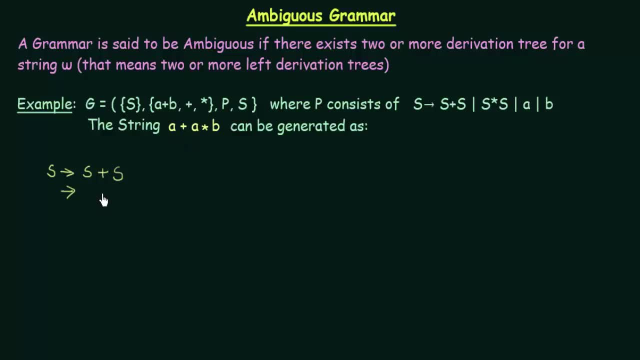 Now, this A is what I need to get, and I am forming the left derivation tree for this. So this is a left derivation tree, So we have to start from the leftmost symbol, which is S. So here, this S, I will replace it with A, because we have a production which says S gives A. 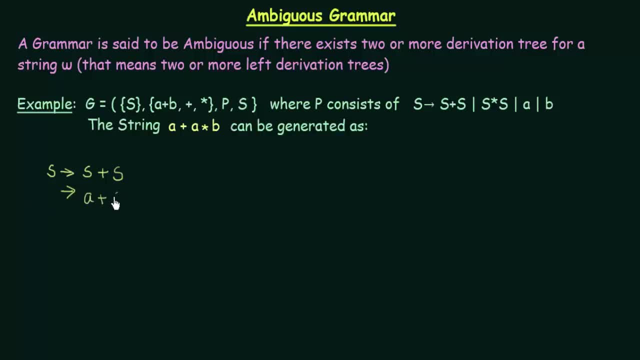 So this S will be replaced by an A and the other S. let me just write it down as it is. And now I got this A plus S and now this A. let me write it down as it is: plus. and I have another S over here and I need A into B. 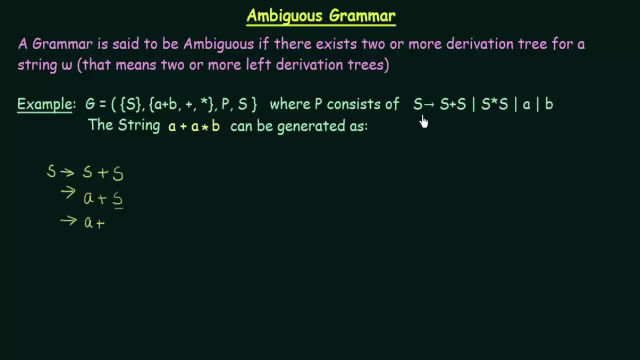 Now let me further expand this S using the production rule, which says that S gives S into S. So this S will be expanded as S into S, and now I will replace this S by A, because we saw that S gives A And I need A in my string. 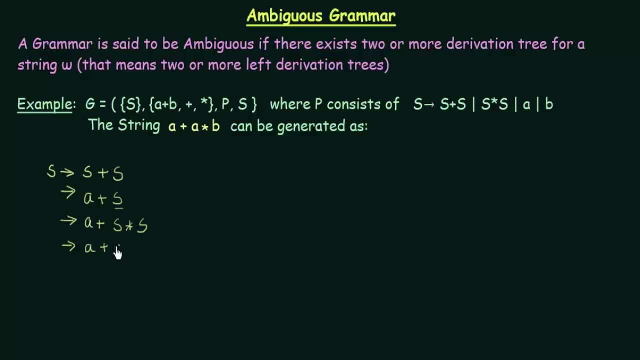 So this A I will write down as it is, and this S, I will replace it with A and into S as it is. And now this final S, I will replace it with B. now I can do that because the production rule says S can give B. 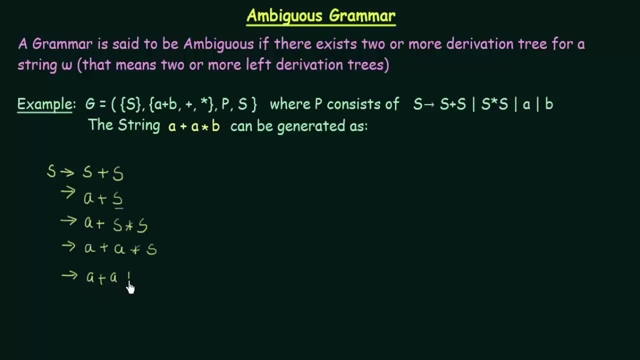 So this A will be as it is. This A will be as it is into this. S will be replaced by B. Okay, so now I am getting the string A plus A into B. Okay, so now I am getting the string A plus A into B. 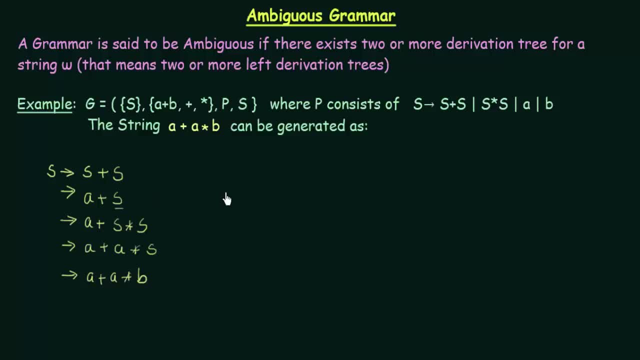 Okay, so this is one way I can generate this string. Now let's see another way in which we can generate. I will again start with the start symbol, And now I will start with the production which says: S gives S into S. 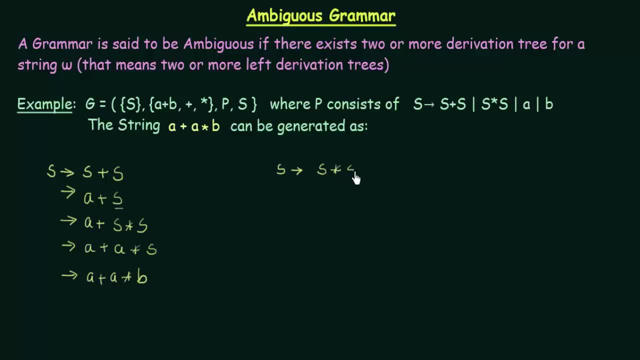 This one S into S. Okay, so this is again a left derivation, So we should start with the leftmost symbol. So here this S, over here. I will replace it with S plus S. S gives S plus S. 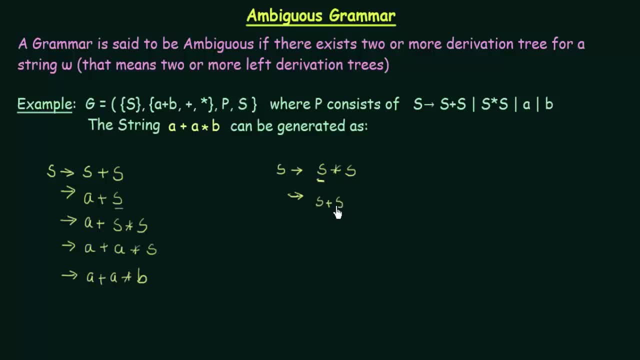 So this S, I will replace it with S plus S, And this into S. I write it down as it is. Okay, so this is what we are getting Now. why am I doing this? This is because I want to get this string. 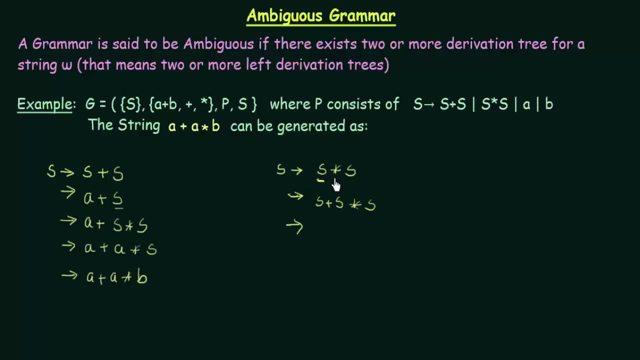 And we see that there is a plus symbol in between and we were having into. So if I do this, I can get the symbol plus. Now I'm having S plus S into S. Now this S over here, I will replace it with A, because S can give A. 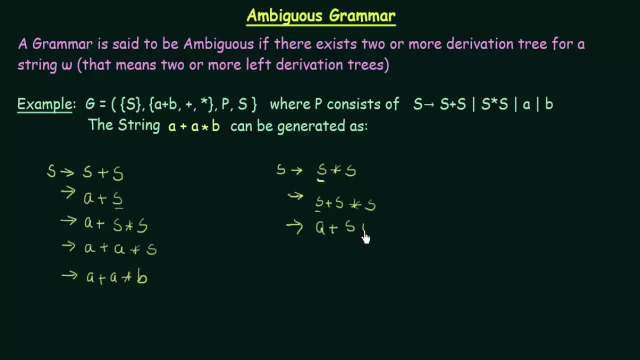 So A plus and this S into S. Let me just write them there, Let me replace this S over here and it will be A again. A plus A into S, This final S. then I will replace it with B, because this S gives B. 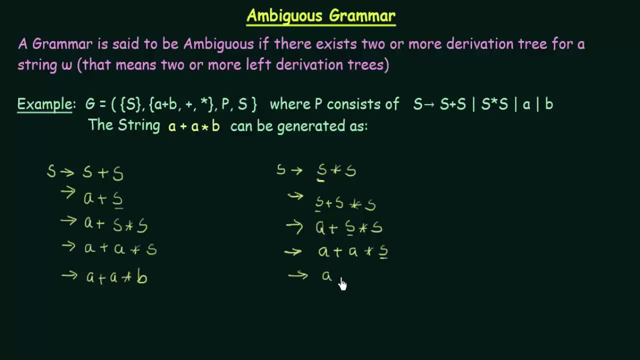 And siguiente: I replace S into S, which gives A. Let's exceed this. give b. So a plus a into b. So now I am getting by string a plus a into b, which is the string I wanted to generate. So we see that this string a plus a into b were generated using two derivation. 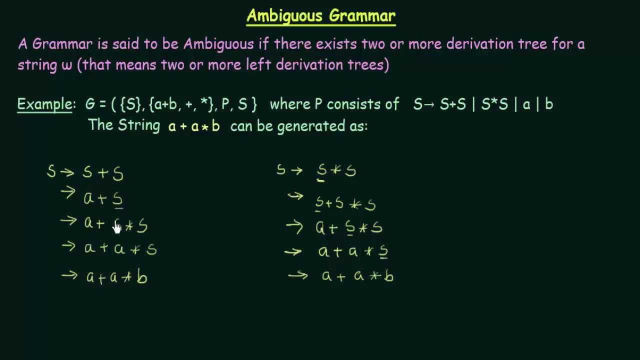 trees. First I chose the production rule s plus s and I could get the string. and even when I chose the string s into s, I could get this string. and we have seen that in both the cases we use the left derivation tree. So, using the left derivation tree, we were able to derive the string in two. 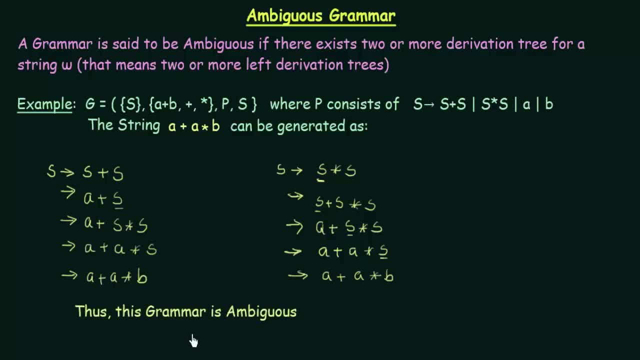 ways. Thus we can say that this grammar is ambiguous. All right, So this is the example of an ambiguous grammar and I hope it was clear to you. So thank you for watching and see you in the next one.